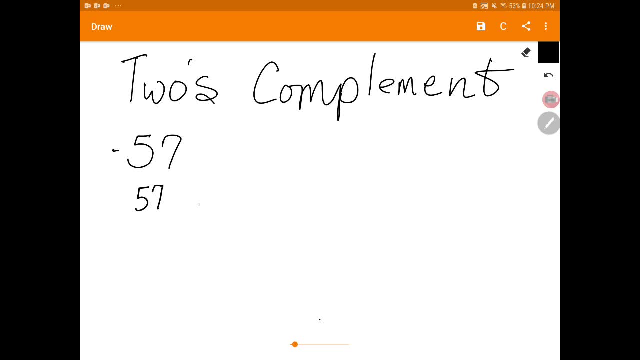 do is we take positive 57 and we're going to draw out eight dashes: One, two, three, four, five, six, seven, eight, And I like to number my dashes. So one, two, four, eight, 16,, 32,, 64,, 128.. 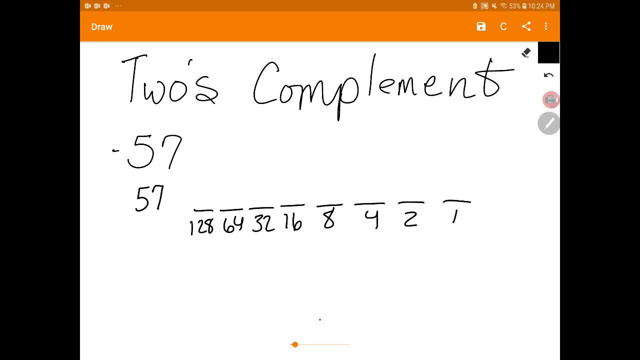 And then we are going to put ones above the numbers that add up to 57 here. So I know we're going to need a 32, and 57 minus 32 is 25.. So I'm going to need the 16,, 25,. 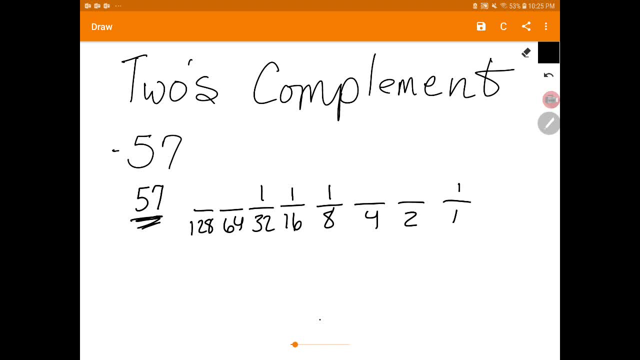 minus 16 is nine, So I'm going to need the eight and the one and everything else becomes zero. Next up, we take the complement of 57. And that just means we take our eight dashes And anytime we see a zero, we turn that into a one, And anytime we see a one, we turn that into. 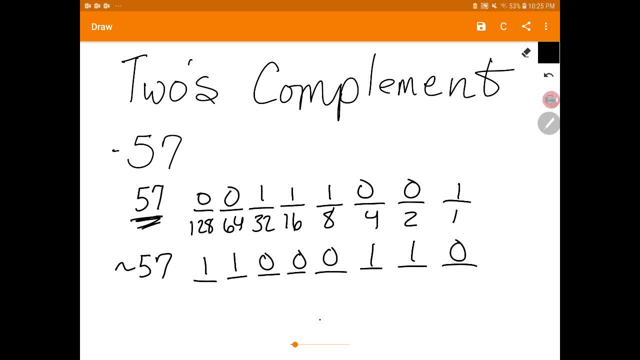 a zero. So we just flip all the bits on the number. Next up we take the complement of 57 plus one. So in that case we add one to our number, And so in this case it's going to be really simple: Zero plus one is one, And then the rest. 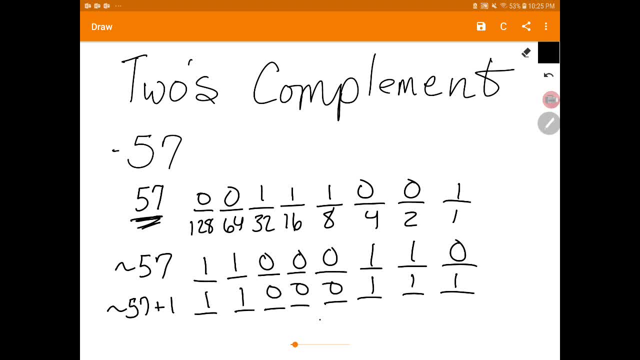 of these numbers are the same. So that's all there is to it. The first thing you do is you figure out the positive version of your negative number, And if your number is already positive, then you just stop at step one. Then we find the complement of the number, and that just means flip all the bits. 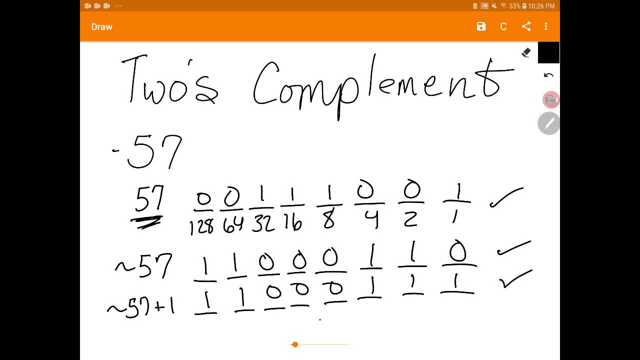 and then two's complement means we add one to that, and that's all there is to it.